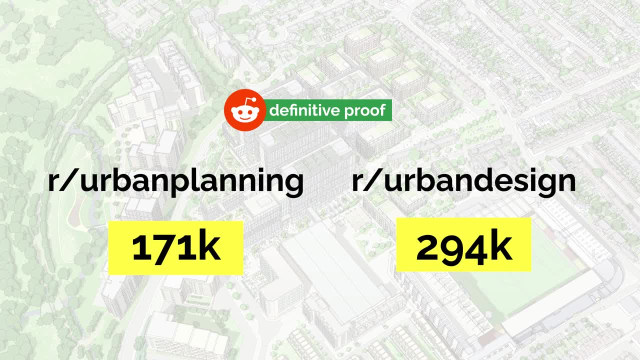 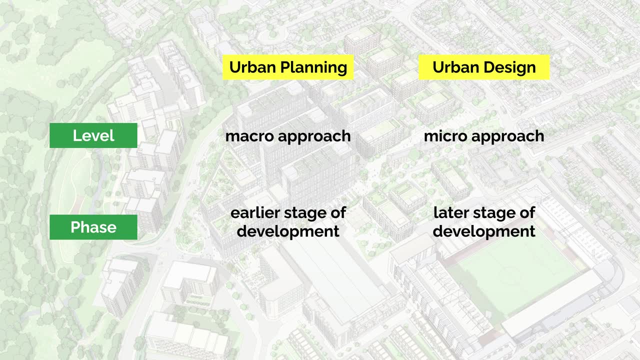 different textbooks and even different subreddits for the two fields. The easiest way to explain the difference between the two is to use levels and phases. Urban planning takes more of a macro approach, focusing on land use zoning and a larger urban vision for 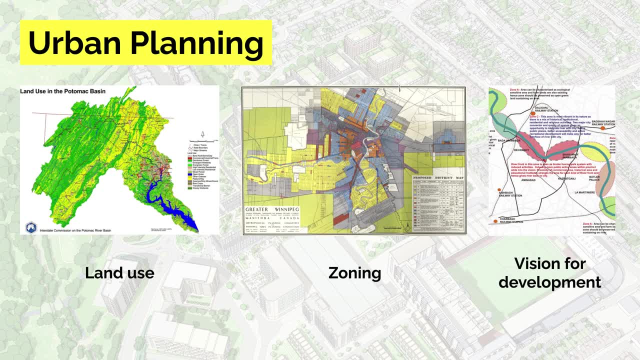 the development of communities. Urban planners use legal documents like comprehensive plans and implementation tools like zoning codes to achieve their vision. Due to the macro approach, urban planning and urban design are not the same. There are different degree programs, different job offers, different textbooks and even different subreddits for the two fields: Urban, 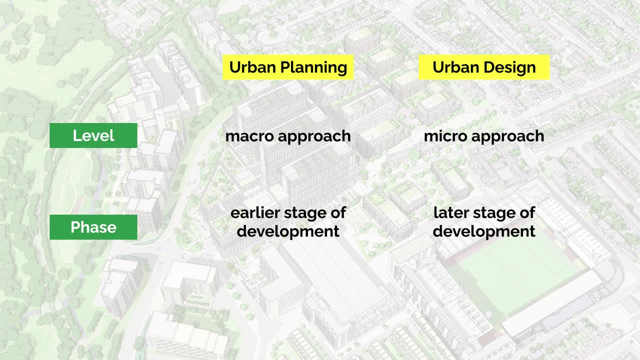 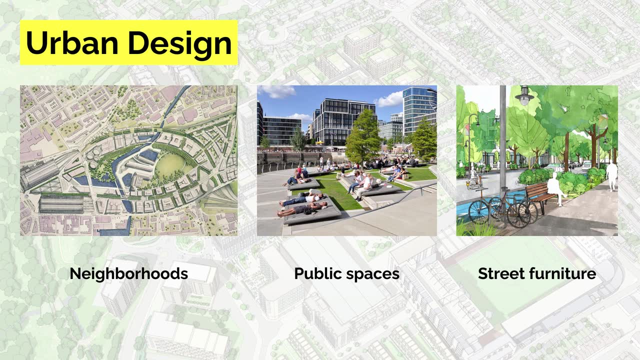 planning takes more of a macro approach. urban planning mostly takes place before the more micro approach of urban design. Urban design concerns the concrete design of groups of buildings, neighborhoods and, in particular, public spaces. It describes the visible and creative aspects of planning. Urban design often goes down to the fine details, like placing street. 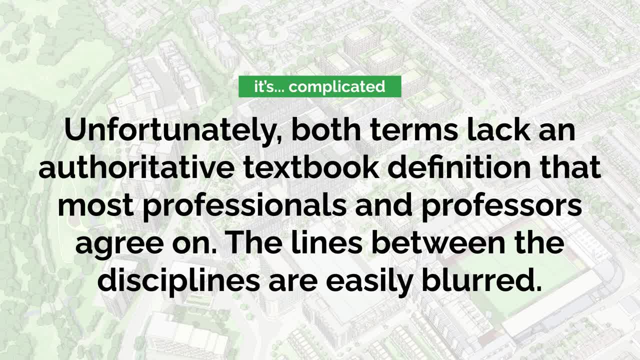 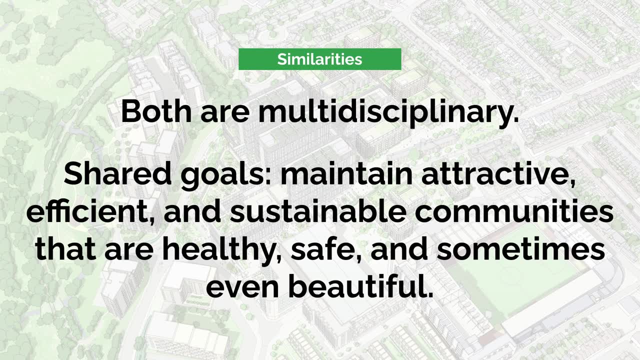 furniture. Unfortunately, both terms lack an authoritative textbook definition that most professionals and professors agree on. The lines between the two disciplines are easily blurred. However, both urban planning and urban design are multidisciplinary fields that share similar goals: To create and maintain attractive, efficient, sustainable communities that are healthy. 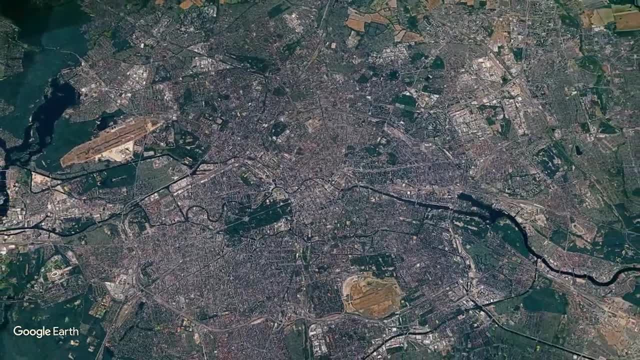 safe and sometimes even beautiful. Thank you for watching. please consider subscribing to help me reach 600 subscribers. 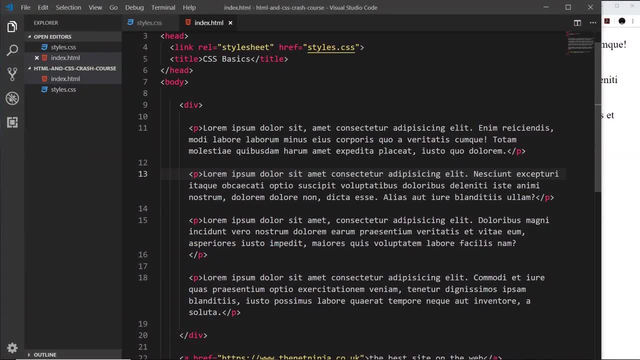 All right then, gang. so hopefully now you have some idea of what CSS is. I hope so, anyway. And now we're going to take it one step further and we're going to talk about selectors a little bit more, and classes and that kind of thing, So we kind of know what selectors already are. 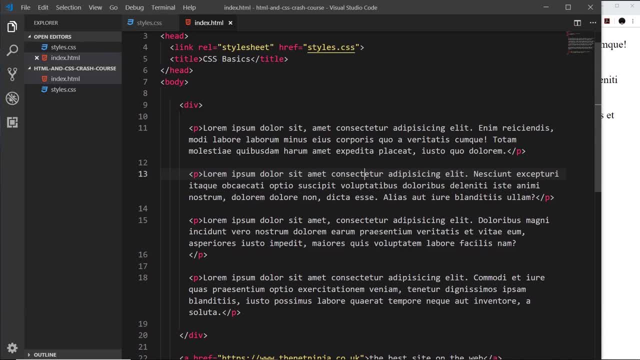 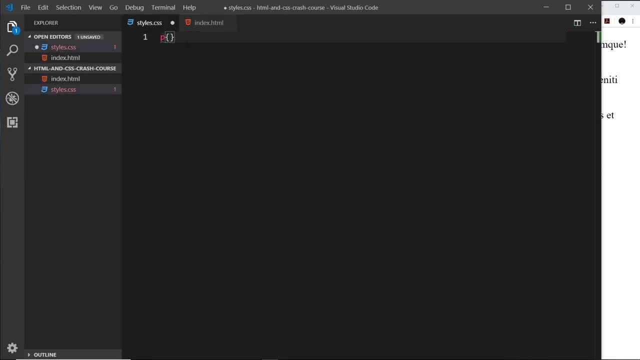 If we want to style something in CSS, we'd create a selector to target a certain thing. For example, if we want to target the p tags, then we would just simply write p and that would be our selector. Then we'd write the declarations inside here.